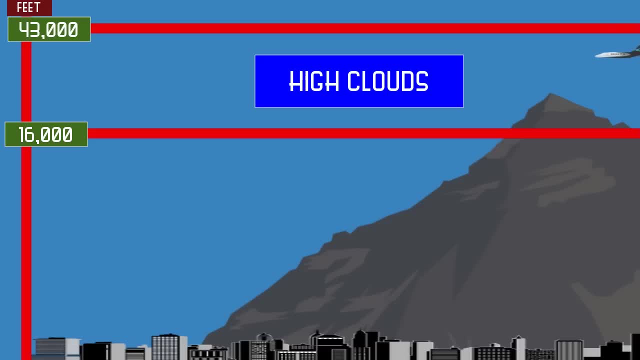 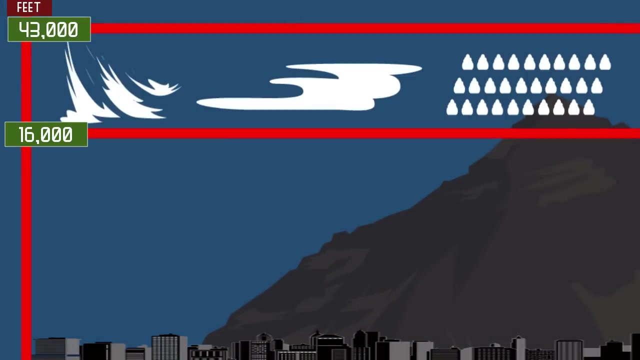 in the middle of the night, On the top of really high mountains or at the cruising altitude of a jet airplane. Due to the extreme conditions at which they form, they tend to be comprised primarily of ice crystals and they do not block sunlight. High clouds include cirrus cirrostratus and cirrocumulus Cirrus. 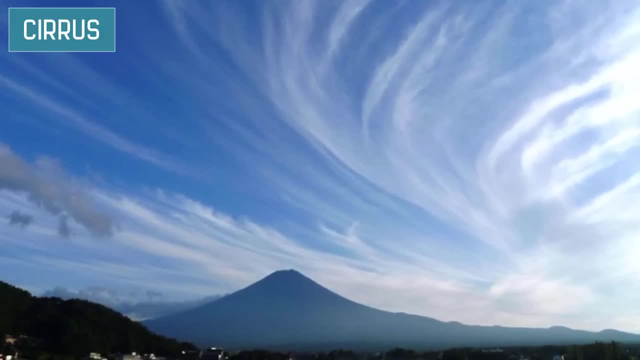 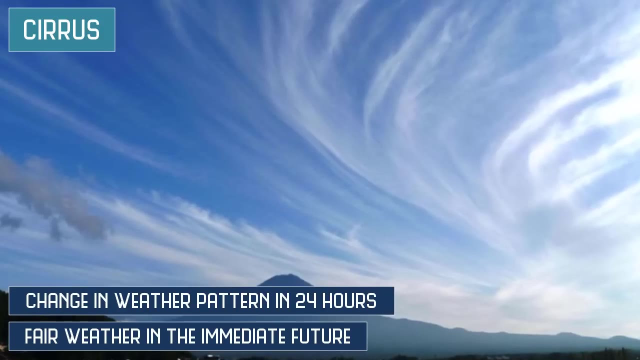 clouds are white, wispy clouds that stretch across the sky. By all accounts, cirrus clouds indicate fair weather in the immediate future. However, they can also be an indication of a change in weather patterns within the next 24 hours, most likely a change of pressure fronts. 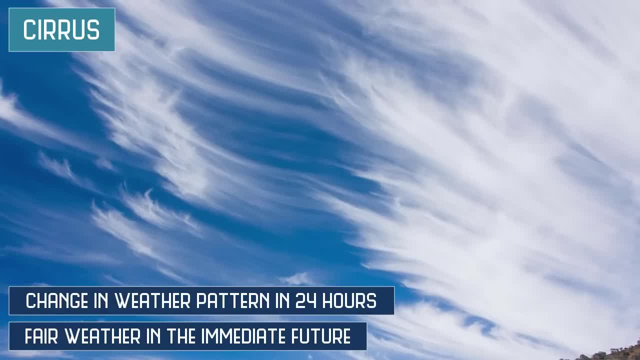 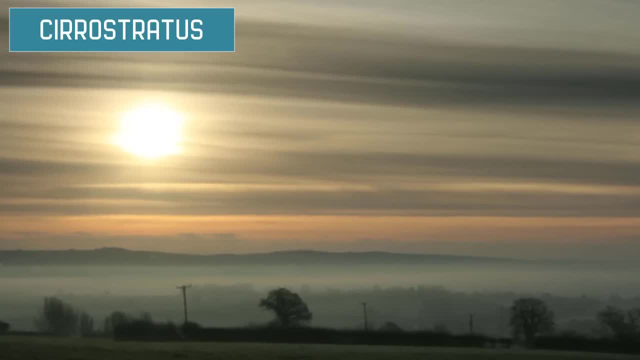 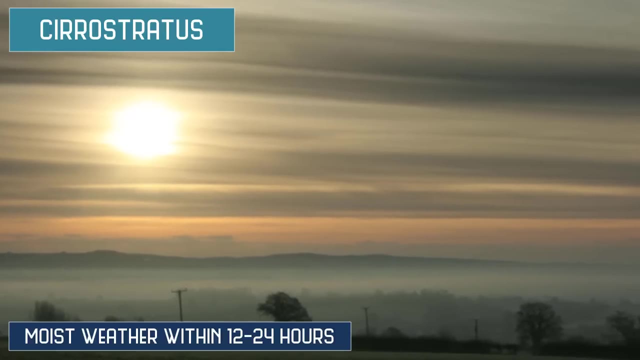 By watching their movement and the direction in which the streaks are pointed, you can get a sense of which direction the weather front is moving. Cirrostratus tend to be sheet-like and cover the whole sky. You can usually tend to see the sun or moon through them. Their presence usually indicates 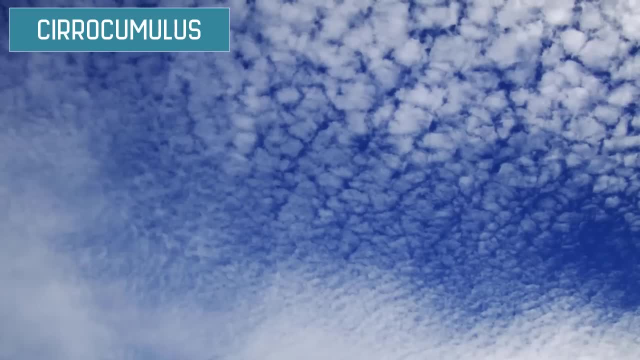 moist weather within the next 12 to 24 hours. Cirrocumulus clouds tend to be large groupings of white streaks. Cirrostratus clouds do not always appear to be covered by a strong speaker In the that are sometimes seemingly neatly aligned. 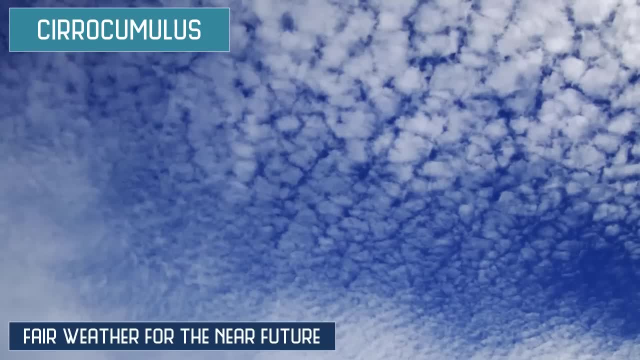 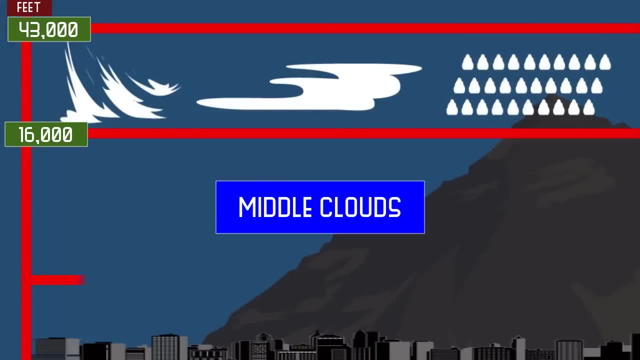 In most climates, these mean fair weather for the near future. However, in the tropics, these clouds may indicate an approaching tropical storm or hurricane. depending on the season, Middle clouds form at 6,500 to 16,000 feet. 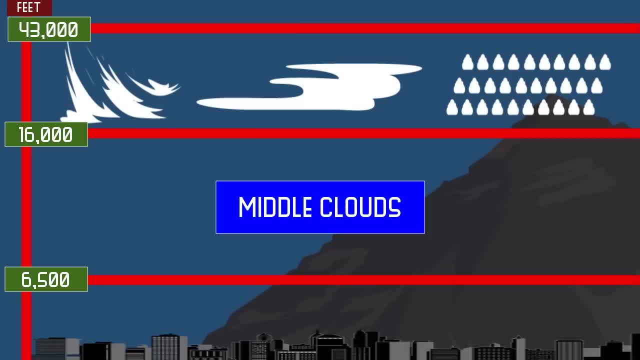 They are comprised of water and, if cold enough, ice, and they often block sunlight, but not always. Middle clouds consist of altostratus and altocumulus. Altostratus are gray and or blue clouds that cover the whole sky. 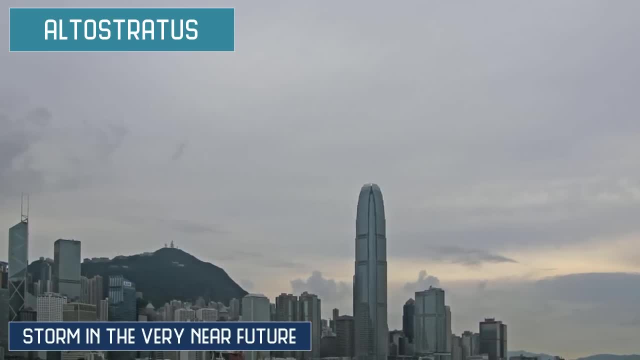 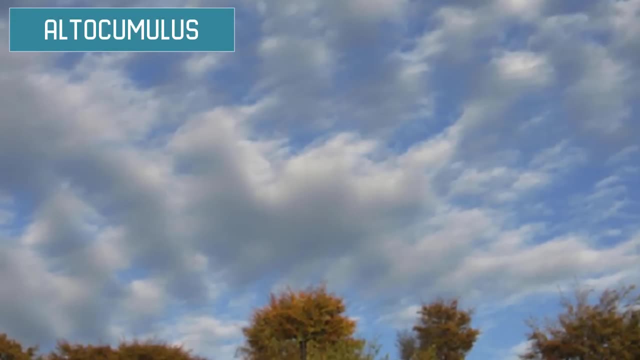 They tend to indicate a storm sometime in the very near future, since they usually precede inclement weather. Altocumulus are grayish-white clouds blanketing the entire sky. They tend to look like large fluffy sheets in which there is a lot of contrast between light and dark. 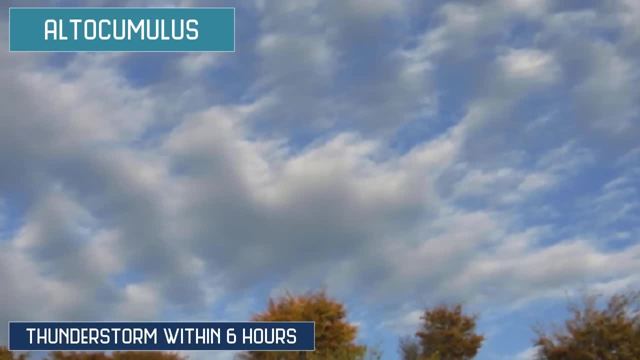 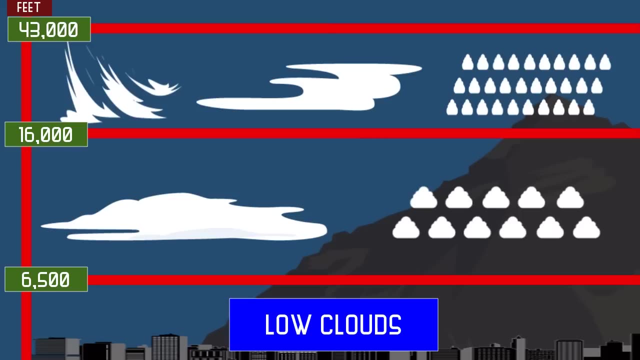 Sun does not pass through them. If you see them in the morning, prepare for a thunderstorm. in the afternoon, Low clouds form at 6,500 to 16,000 feet. These clouds are the ones that like to hang around just above tall buildings. 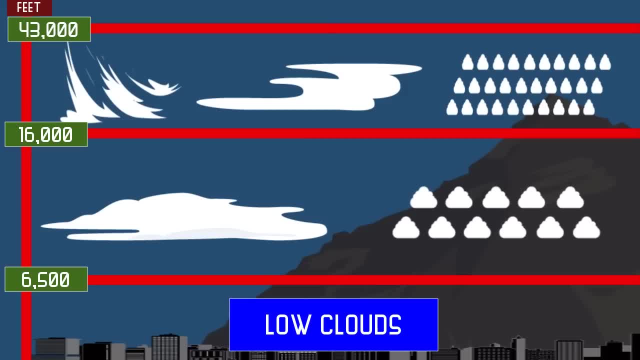 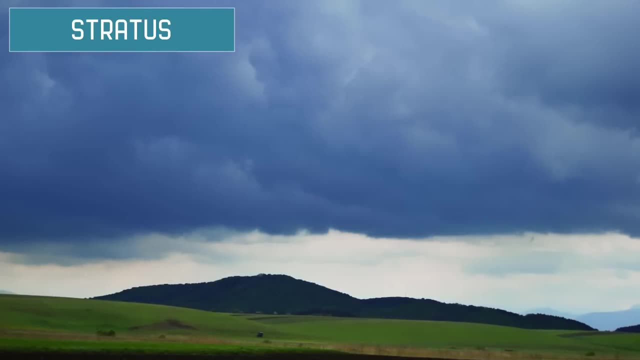 These clouds tend to contain water, but can also be comprised of snow, if the weather gets cold enough. These clouds block sunlight and can bring precipitation and wind. Low clouds include stratus, stratocumulus and nimbostratus. Stratus are low-lying solid clouds that are often formed. 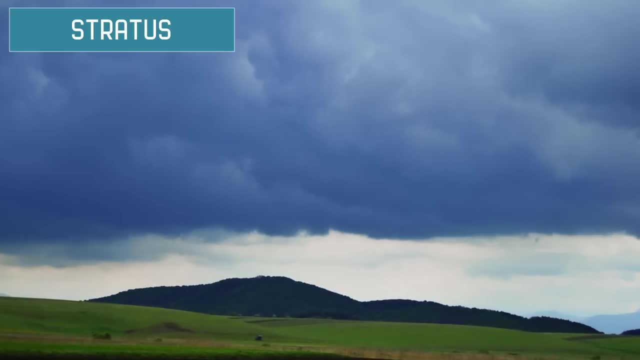 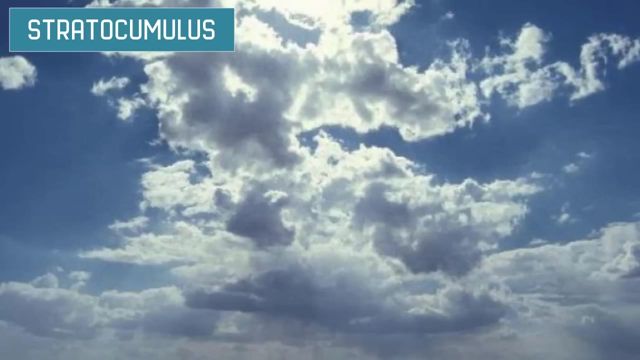 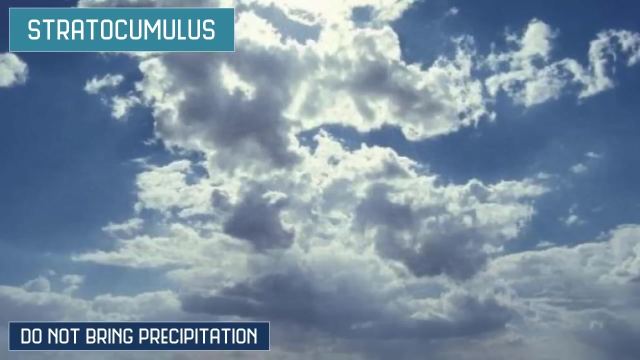 when fog lifts off the ground. These clouds obviously look like an elevated fog. Often they bring drizzle or light snow. Stratocumulus are low-lying, bumpy and gray clouds. They do not bring precipitation. They also do not cover the entire sky and tend to come in rows and patches. 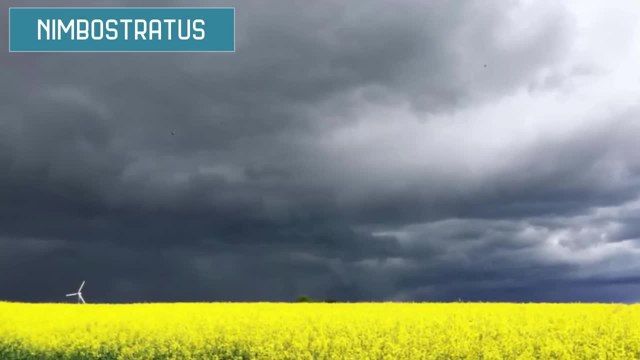 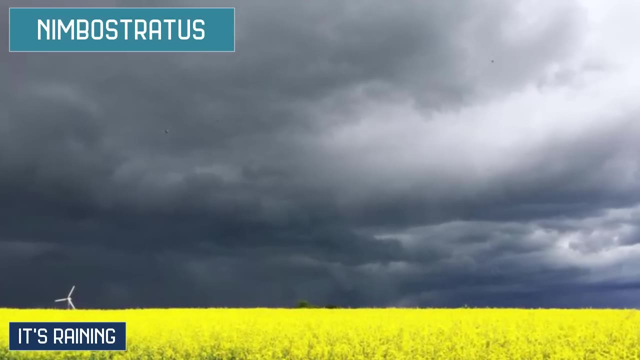 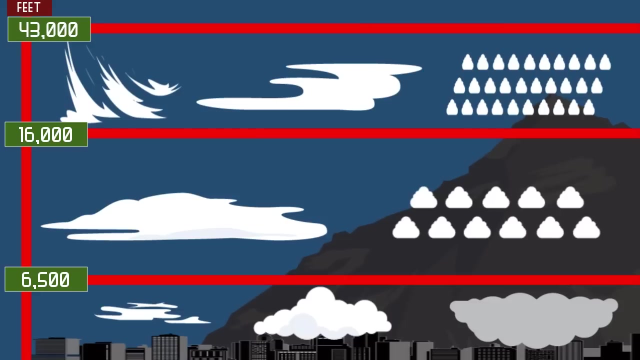 Nimbostratus is your standard rain cloud. It is a large flat sheet of gray cloud with a little bit of differentiation. If you see these, chances are it's raining outside. Not least are clouds with vertical growth, which tend to have a base that hangs really low, around 5,000 feet. 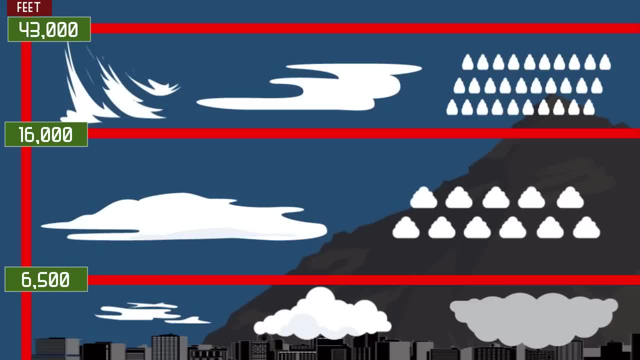 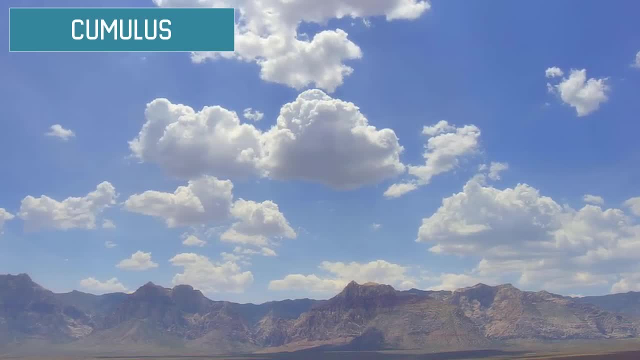 and a top that climbs really high, over 50,000 feet. Clouds in this category include cumulus and cumulonimbus. Cumulus clouds are your stereotypical white cotton ball clouds. So long as the clouds remain low, clumps floating across the sky. 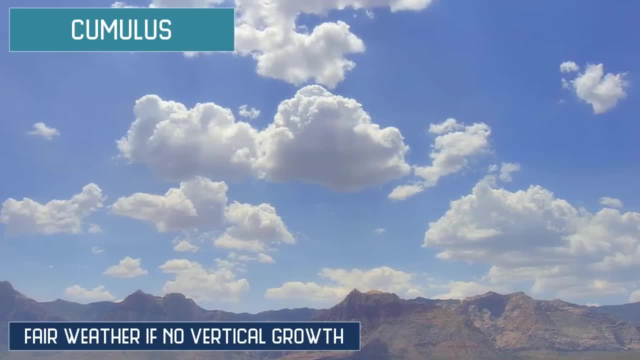 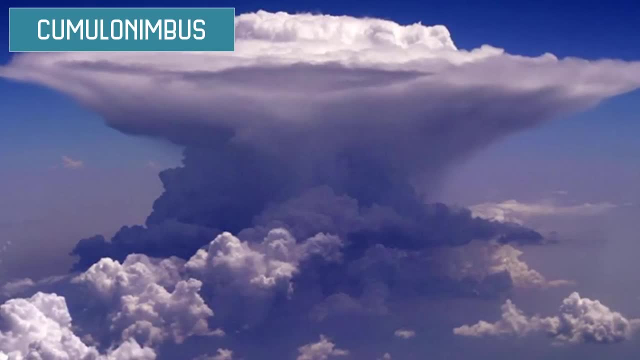 there will be fair weather. However, you need to keep an eye on these clouds, as any vertical growth can indicate the start of a large storm. Cumulonimbus are cumulus clouds that have grown vertically into an anvil-like shape. The anvil tends to point in the direction the storm is moving. 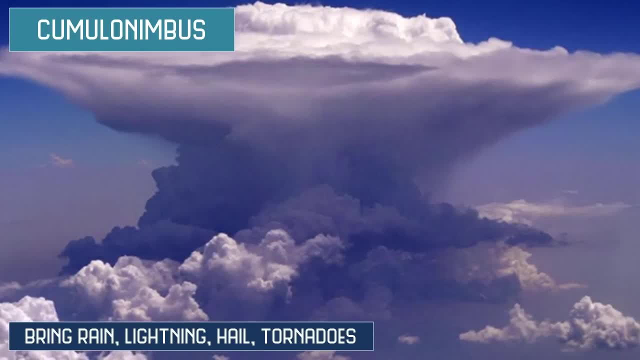 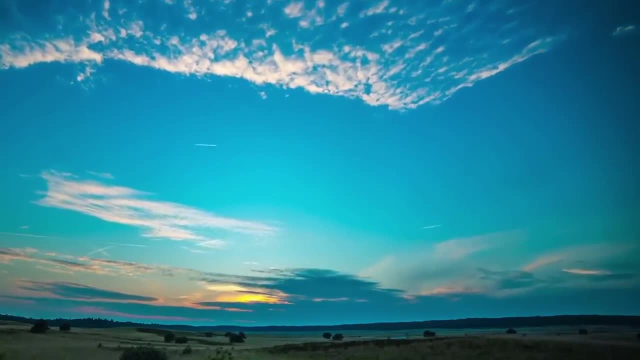 These clouds bring most dangerous weather, such as rain, lightning, hail and tornadoes. Alright, now that we know what the basic types of clouds are, we need to look up at the sky, Go outside and look at the sky. If there are no clouds in the sky, then the weather is fine. 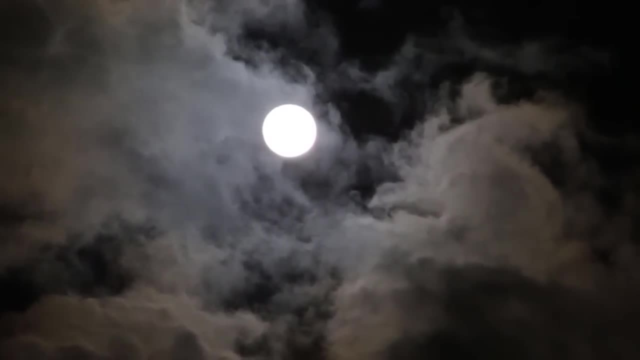 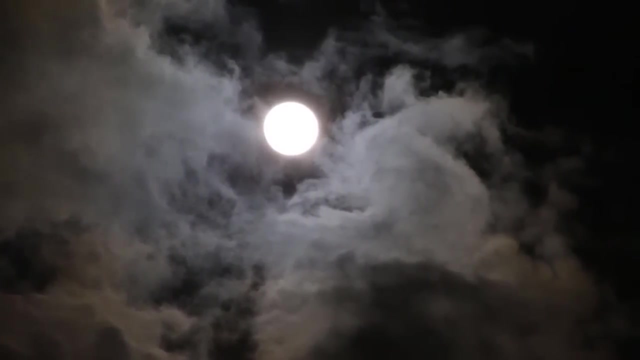 Assuming there are clouds in the sky, we now need to identify them First. determine if you can see the sun or moon through them. If you can, then you are looking at high-altitude clouds. If the clouds are thick, then there is a chance of poor weather a day or two in the future. 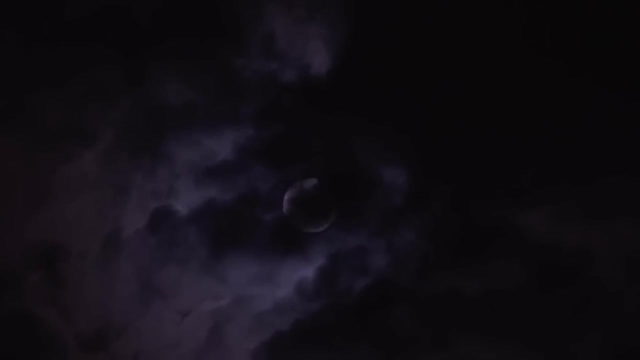 To determine when the storm will arrive, observe whether or not the clouds appear to be moving. If they appear stationary, it is a slow-moving front and probably won't arrive for over a day. If they appear to be moving, then the change in weather will be there faster.